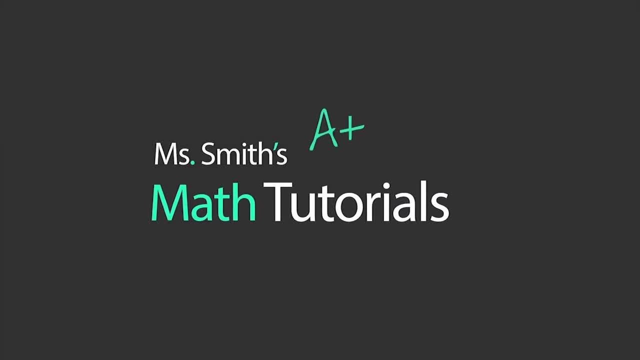 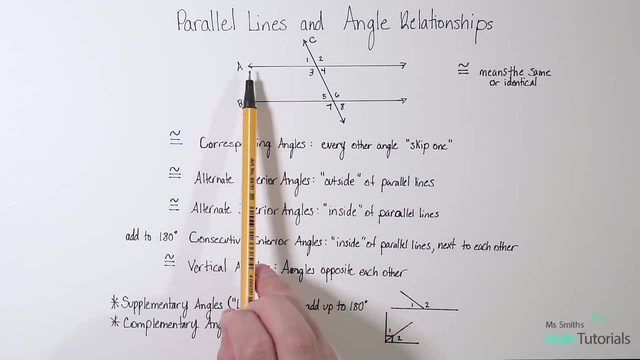 Welcome to Ms Smith's Math Tutorials. I'm Ms Smith. In this video, we're going to be talking about parallel lines and angle relationships. A couple things we want to establish is that A and B have to be parallel lines in order for these to work. So this is operating under the. 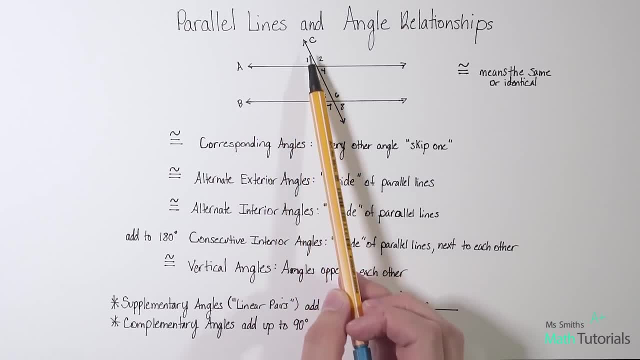 assumption that A and B are parallel. This cut-through line is called a transversal, this C line. He is cutting through two or more parallel lines and it creates these angle relationships and we're going to talk about those. One thing that we do need to establish: 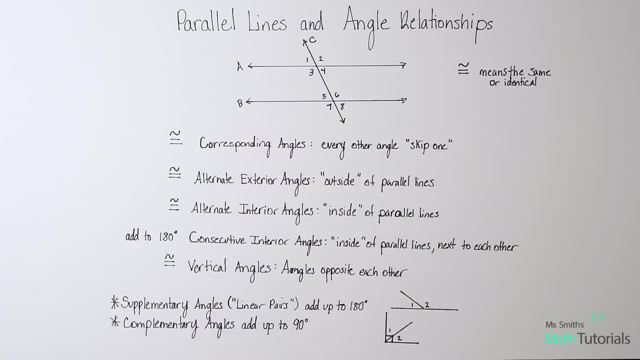 is this symbol? This means congruent and it's essentially an equal sign, but we use it specifically when we're talking about shapes or angles or triangles and all that stuff. So this means congruent, It means the same, or identical, or equal. 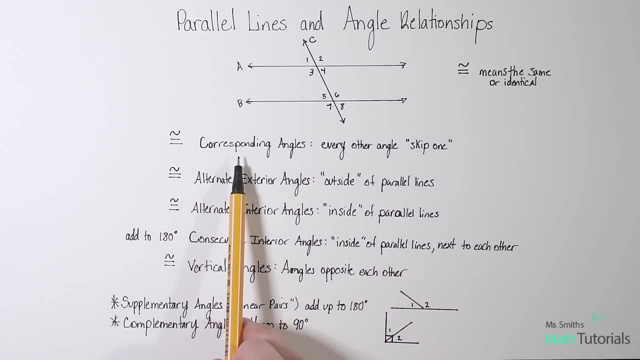 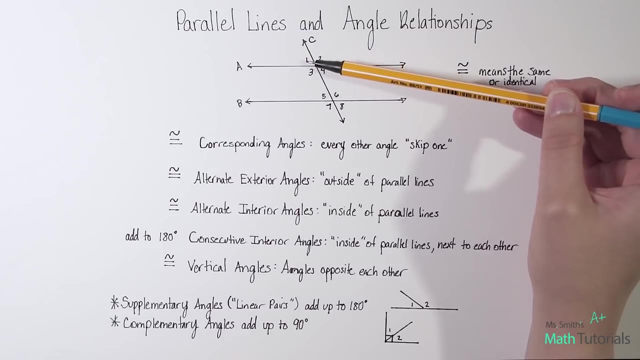 The first type of angles that we're going to talk about are corresponding angles. The easiest way I can sum it up is: you pick an angle and then you skip one and you go to the next angle. Let me show you what I mean: Pick number one, skip number three, go to number five. So one and five. 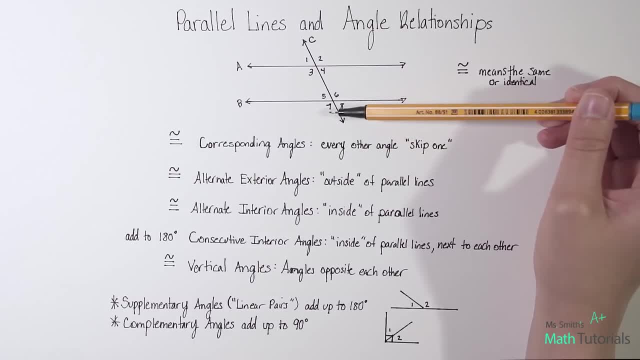 are corresponding angles. I could do the same thing with seven. I could say: all right, I pick seven, skip five, go to three. Seven and three are corresponding angles. I could do the same thing with seven, and three are corresponding angles. So we just laid out two of them, so let's write. 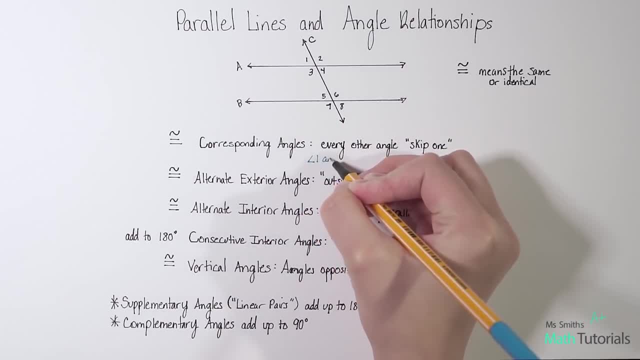 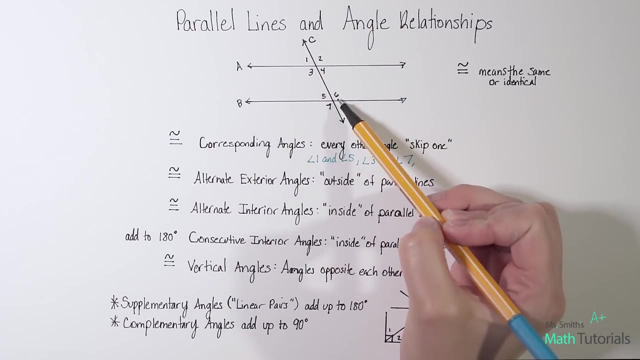 those. We've got angle one and angle five, and then we said angle three and angle seven. What else could we get? We could do: angle two, skip four, go to six, So angle two and six. So eight, skip six, go to four, So eight and four are corresponding angles. Angle eight. 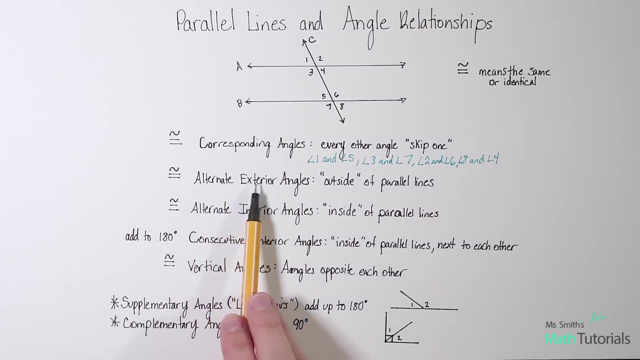 Our next type of angle that we're going to talk about is alternate exterior angles, And I should know- I don't know if I mentioned this when I was up here, but corresponding angles are congruent, So that means that angle one, whatever the value is for. 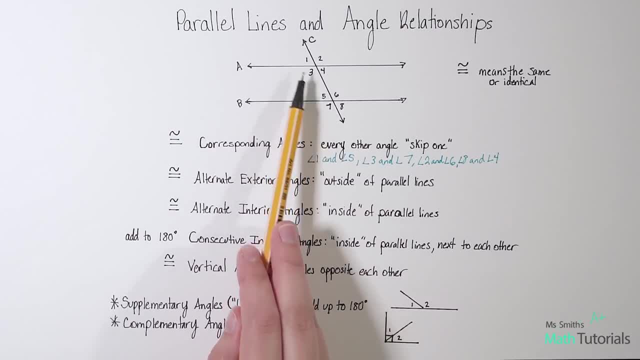 angle one, whatever the measurement is, angle five will be equal to that because they are corresponding angles. So I want to make sure I make that very clear. For alternate exterior angles, these angles are also congruent to each other. They are equal to each other And the easiest way. 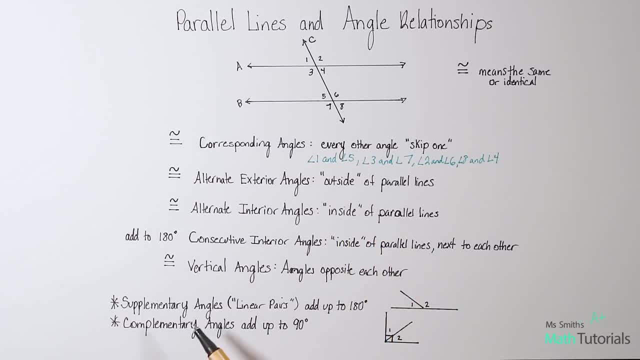 to sum it up is they are outside of the parallel lines. So let's think about it: If our parallel lines are here and here, the outsides would be seven and eight and one and two. These four right here, they would be inside the parallel lines. These are outside, So alternate. 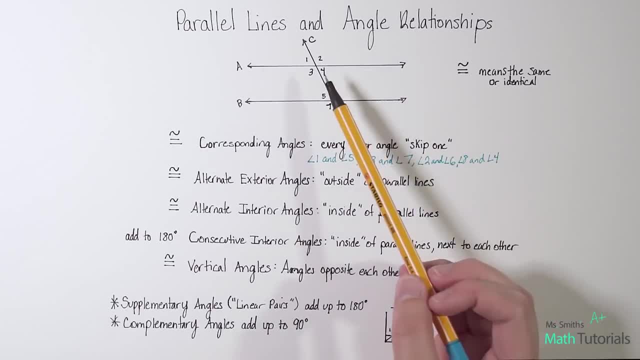 means switching sides, if you will. So one would be an alternate exterior angle with eight. They're on opposite sides of the transversal. We've got one angle one and angle eight, And then we also have alternate exterior angles, Angle two and angle seven. All right, Next we have 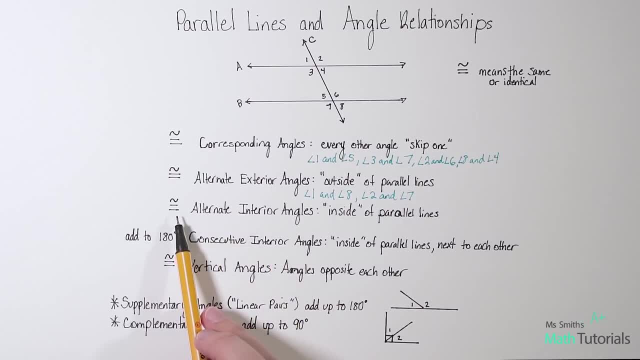 alternate interior angles. These angles are also congruent with each other. They are the same measurement, the same number of degrees. So these are inside, like interior means inside, inside of parallel lines. So if our parallel lines are A and B are inside angles. 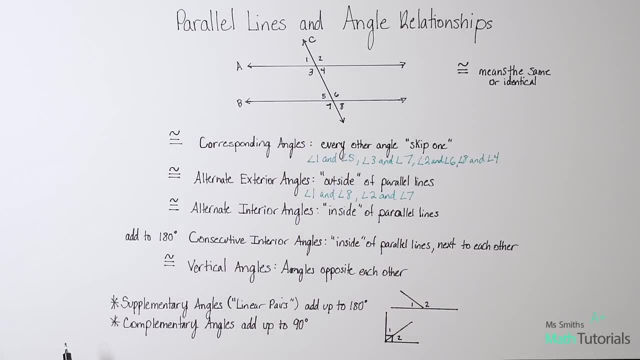 are going to be the three and the four and the five and the six. And again alternate means we're switching sides, We're going the other side. So we could start with three and go the alternate side down here in six. So three and six would be alternate interior angles, So angle three. 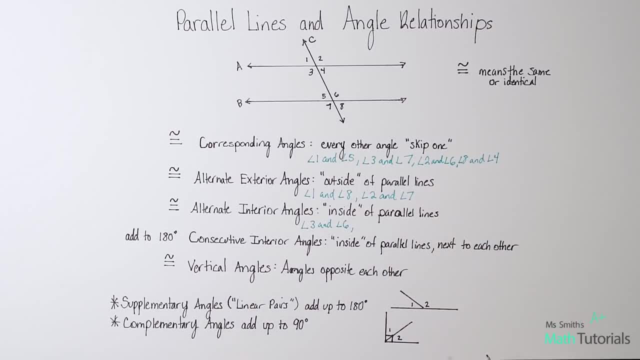 and angle six, And then our other alternate interior would be angle four and angle five. All right, Our next type of angle is consecutive interior angles. Okay, So these are inside of the parallel lines, similar to the alternate interior angles. They are also inside. 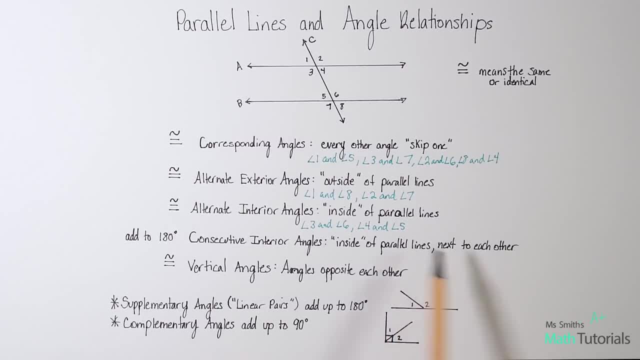 but these are next to each other, So meaning three and five would be consecutive interior angles. We're not going alternate, We're not switching to the other side, We're going consecutive straight down. So three and five would be one angle, three and angle five And then the. 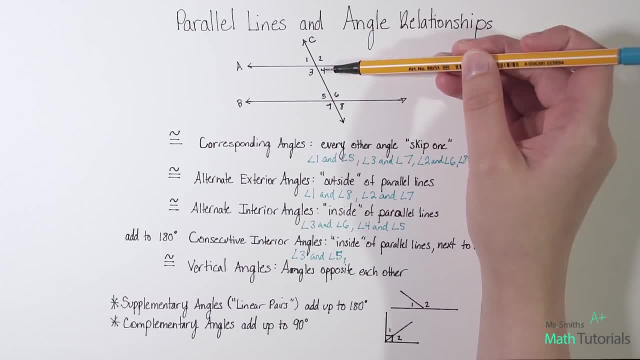 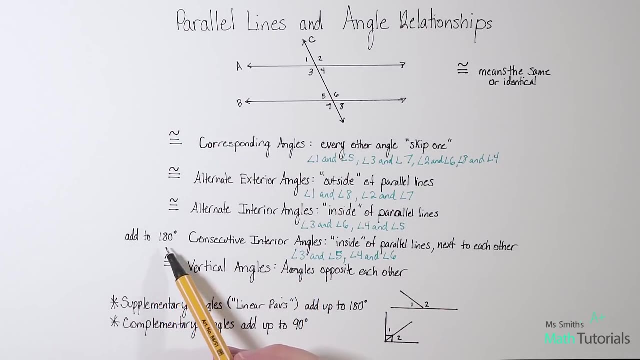 other one. the other consecutive interior would be angle four and angle six, So right beside each other, And an important thing to know about consecutive interior angles is that they do not. they're not congruent with each other. Okay, And I can even look at three. I see this is clearly. 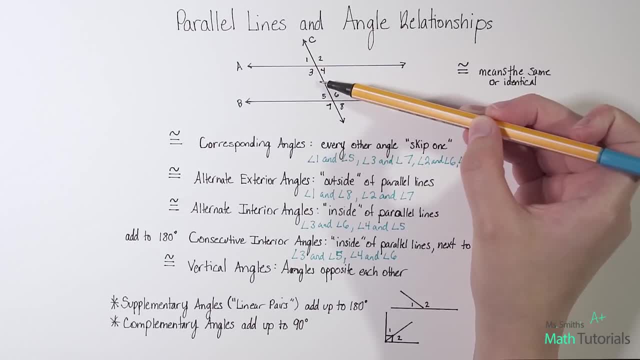 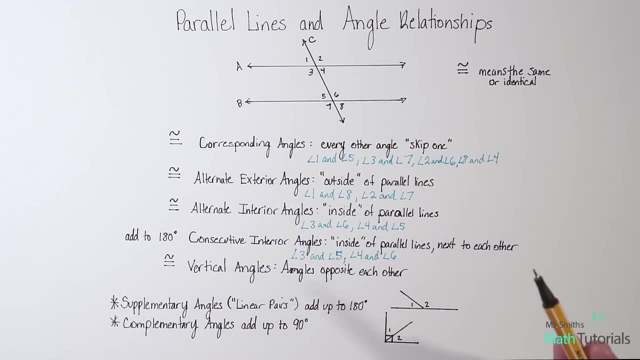 an obtuse angle. It's larger than 90 degrees, And this five it's clearly an acute angle. It's less than 90 degrees. So I can just look at those and tell those are absolutely not congruent. But what do I know about them? They add to 180 degrees. Okay, So 180 degrees, that's going to be a big. 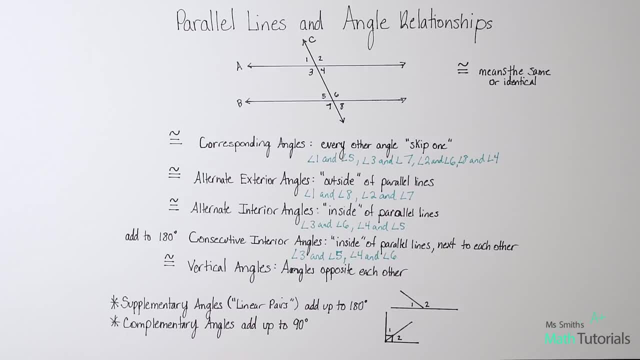 number that we work with a lot And then we're going to add to 180 degrees. So we're going to go through our angles and triangle units, So you want to get used to that number. But consecutive interior angles add to 180 degrees. Our next angle is vertical angles. So these are 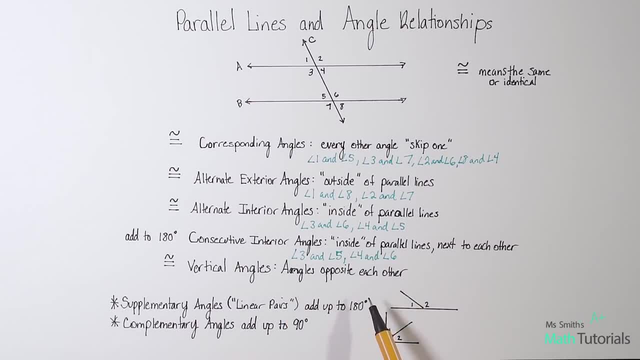 angles opposite each other. So I kind of think of them as like the X angles. Okay, So for example, one is opposite, with four right Angle one and angle four, And you see how it creates like an X shape. So on one side of the X is one and on the other side is 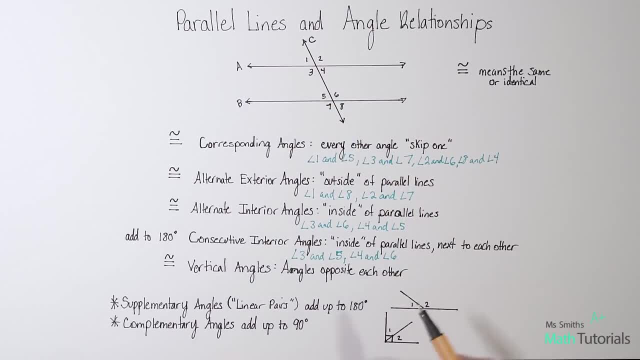 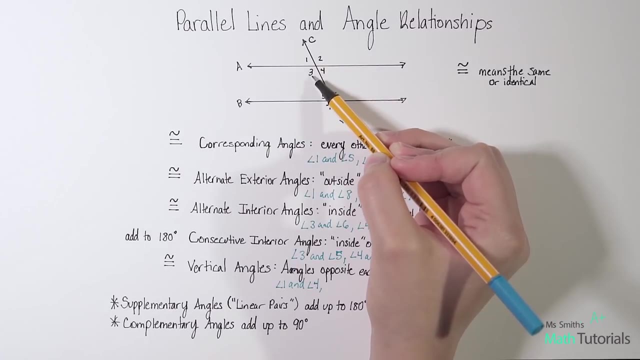 four. Those two angles are congruent with each other, So we've got angle one and angle four. Okay, Let's see what else in that same X right that we've created, I could see. angle two and angle three are directly opposite each other, So those are also vertical angles. 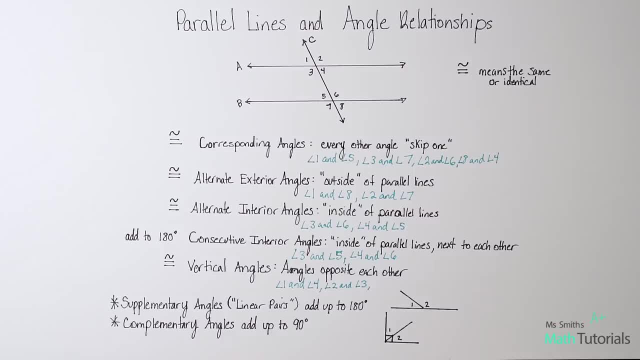 Angle two and angle three. Looking down here, we could go with five and eight. Those are vertical angles: Angle five and angle eight. And then our last one would be angle six and angle seven. Those are also straight across from each other and they are congruent: Angle six and angle seven. 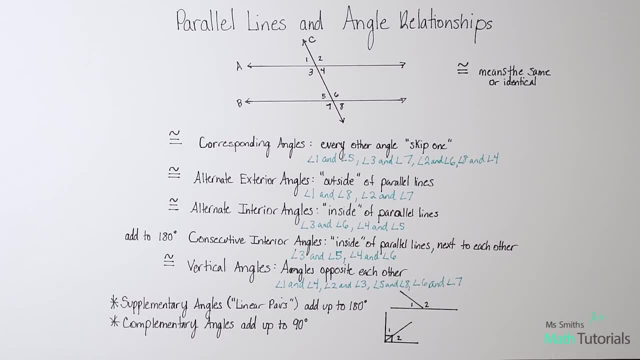 Okay, Two other terms that you're going to hear. So I just want to level the form out of this, because even right now I'm kind of lacking theenger than I'm supposed to have. So I just want to lay out right at the beginning what these terms mean. 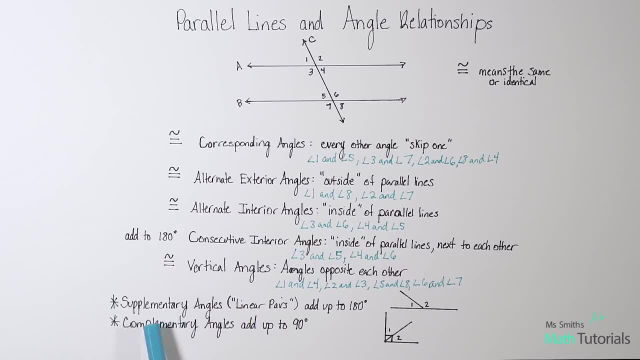 The first one. you're going to hear a lot in both of these forms: Supplementary angles, linear pairs. Those are angles that add up to 180 degrees. An example here that I've drawn, just a rough sketch of a linear pair. Notice that one and two are on one side of a straight line. 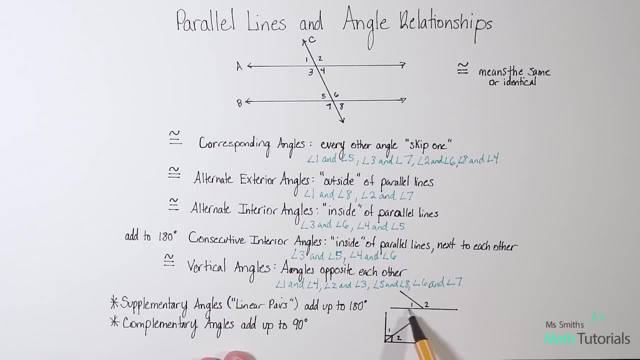 And we are assuming that that is a perfectly 180 degree straight line And even though it's cut into two angles, one and two- if I can draw a little rainbow half circle like that, then that means this is a linear pair, They're supplementary angles and they add up to 180 degrees. 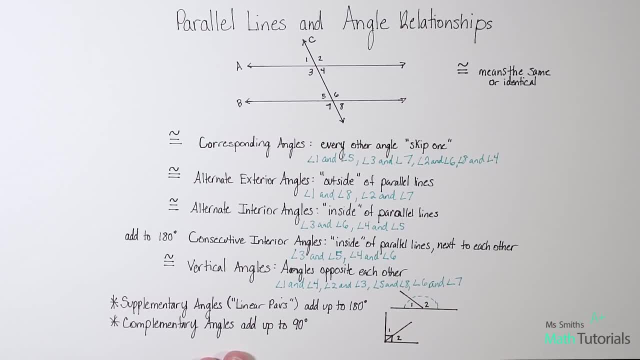 So that's something that's really going to come in handy when we start doing more stuff with triangles and different, you know, almost puzzles, trying to figure out what angles are what values. This is going to be a really helpful tool If you can identify those straight lines and the linear pairs. 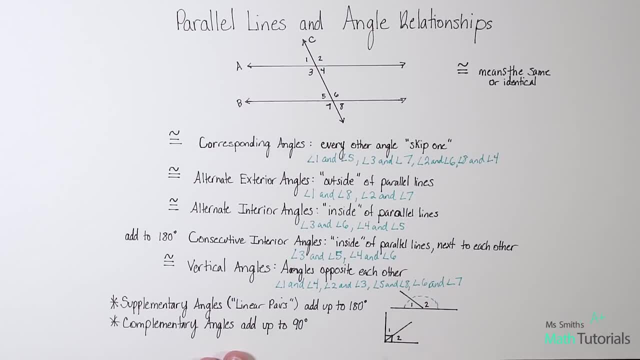 that can help you determine what those angles are. So the other term I want to talk about briefly is complementary angles. So this we won't see as much in our units but it will pop up every now and again. So if two angles or two or more are complementary, 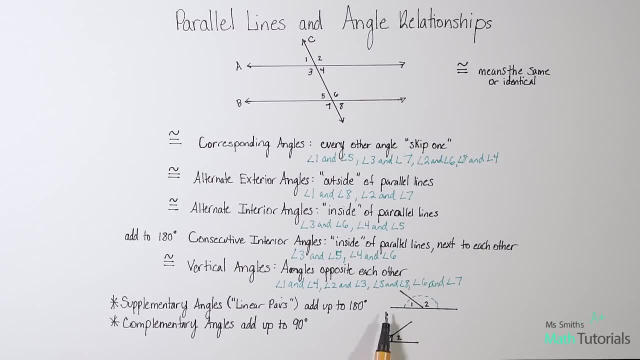 that means they add up to 90 degrees. So an example here you can see this is a 90 degree angle and it's marked with that little box which means that's math language for it, That is a 90 degree angle. 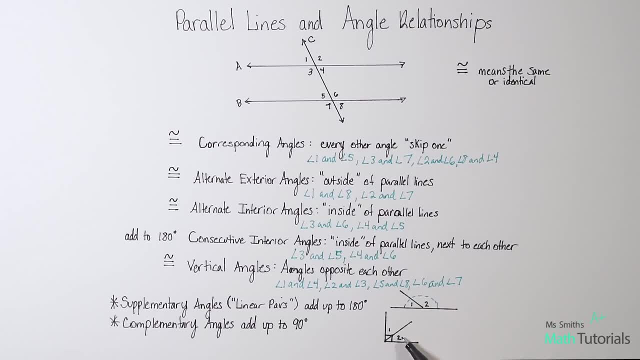 Okay. so, even though it's cut in two, I know that one and two, if they are complementary, they will add up to 90 degrees. Let's look at some examples of different angles and identifying. Okay so let's look at some examples of different angles and identifying. 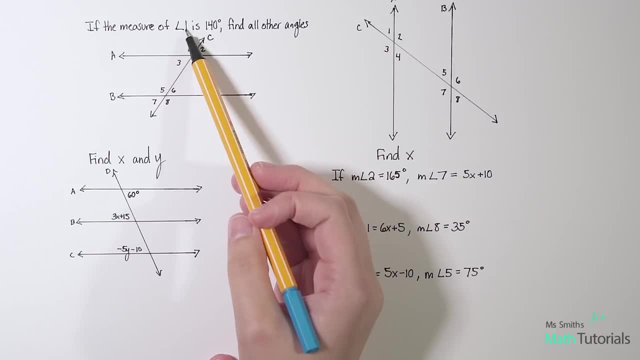 So here's the first one. If the measure of angle one- okay, angle one right there- is 140 degrees, find all other angles. Now that may seem like a daunting task. You may think I don't have enough information to do that. 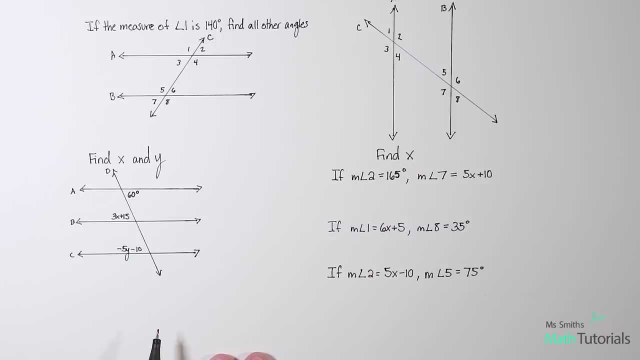 But if we just follow those rules that we went through on the first page, we can actually identify every single one of these angles, just by knowing one of them. Again, we are operating under the assumption, And the assumption is, I'm telling you that A and B are parallel to each other. 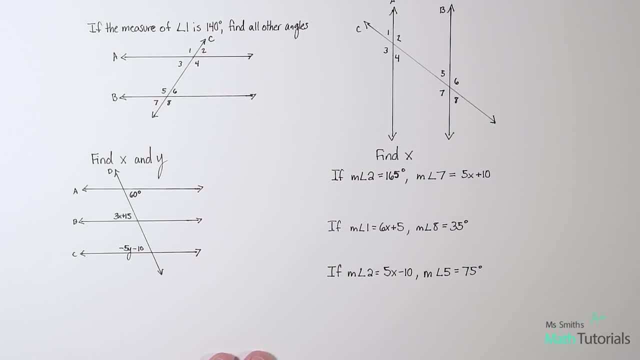 And C is a transversal that cuts between them. We are operating under that assumption. Let's go ahead and measure what angle one is. So it told us one is 140 degrees. So I could go a number of different ways from here based on those rules. 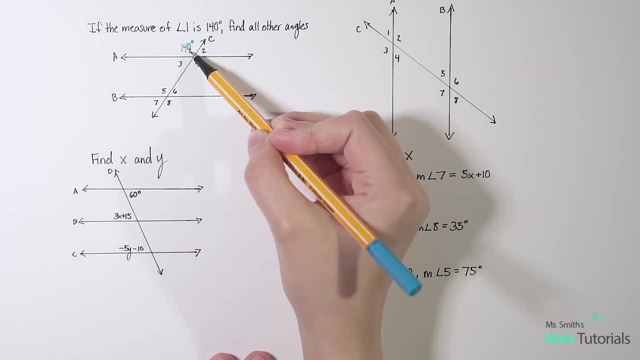 But the first one that sticks out to me is: if one is 140 degrees, then so is four, Because those are vertical angles, They're directly across from each other And I know vertical angles are congruent. So I know four is also 140 degrees. 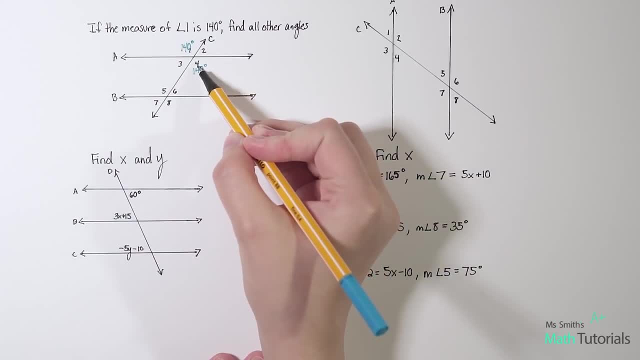 All right. Now from here I could say: well, four is an alternate interior with five right. They're on opposite sides of the transversal, They're both on the interior of the parallel line, So I can say five is also 140.. 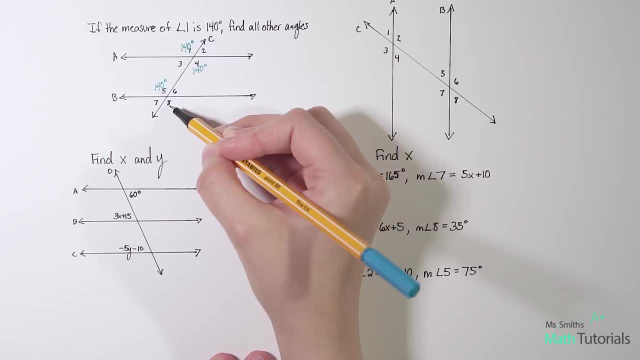 And then from five I could say: well, five is a vertical angle with eight, So vertical angles are congruent, just like we did one and four, So I can say eight is also 140 degrees. OK, so I filled in all my 140 degrees, but what about two, three, six and seven? 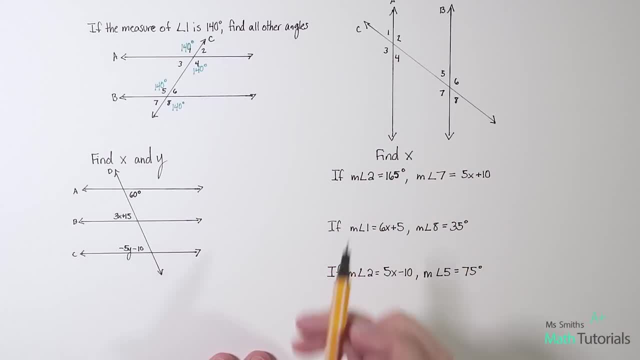 Well, there's lots of different ways I could have purchased, but I'm going to go with. I see, right here I've got this nice straight line Right. So that tells me when I have a straight line and then some angles split between it. 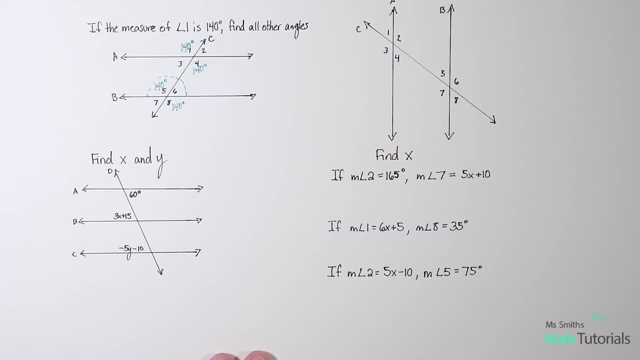 I know that those angles have to add up to 180 degrees. They are supplementary, They are linear pairs. Five and six are currently linear pairs. So if I know that this line has to add up to 180 and angle five is 140.. 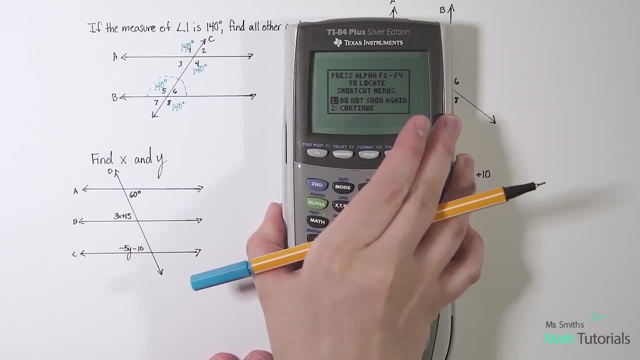 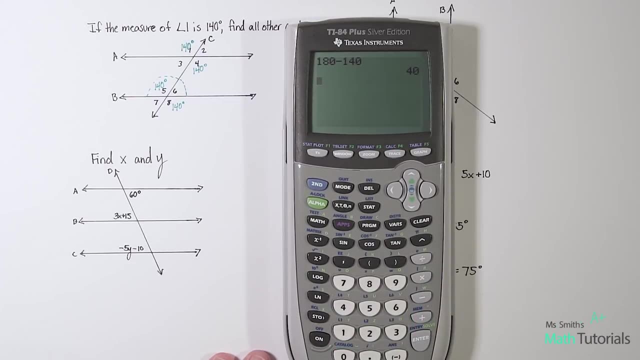 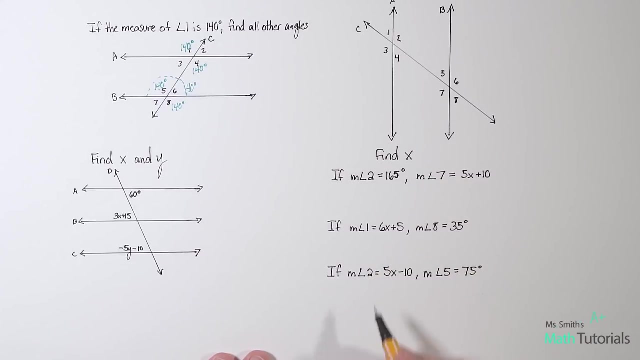 Well, let me get out my calculator: 180.. Minus 140.. Well, that gives me 40 left over. So that tells me that six has to be 40 degrees. And now, if six is 40 degrees, six is vertical angle with seven. 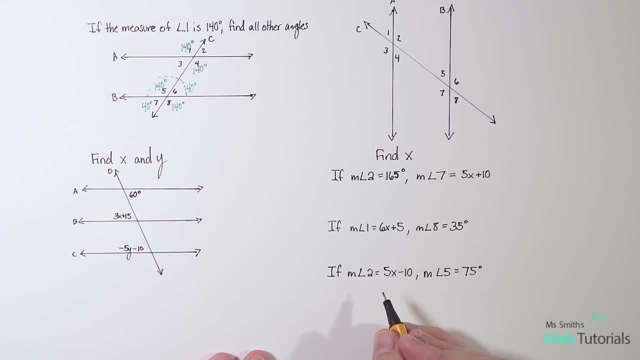 So seven has to be 40 degrees And I could say that angle seven and angle three- remember our pick one, skip one, go to the next one- are corresponding angles That are Congruent. So if seven is 40 degrees, so is three. 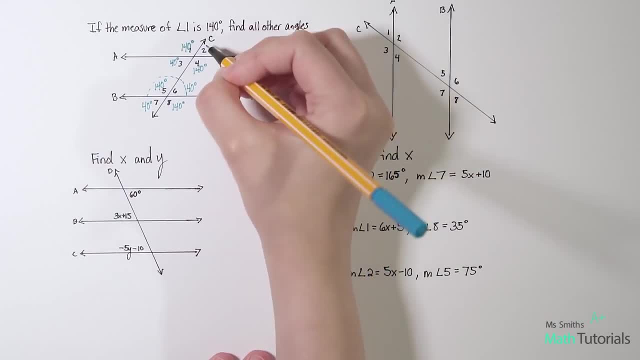 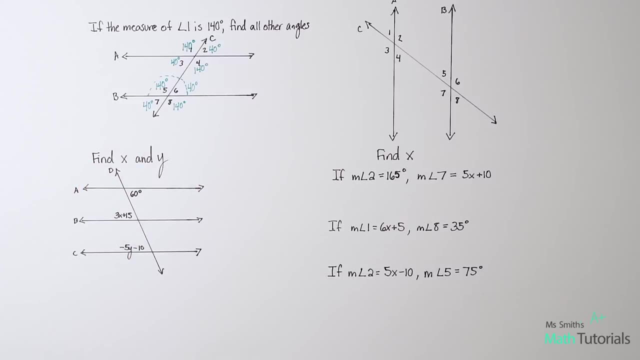 And then three is vertical angles with two, which means two has to be 40 degrees as well. Okay, So you see, if we just know one, in a situation like this we can pull out every single measurement of each angle. Let's look at this one. 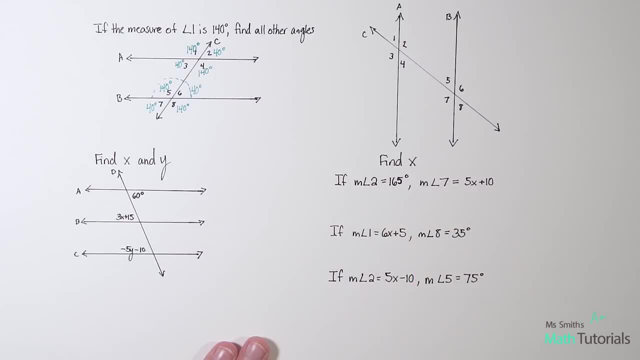 So it's given me a picture and then it says find X For Each of these questions. Now I should note that these questions are all independent of each other, meaning you know, if it tells me measure of angle two is 165 degrees, that's just for that one problem. 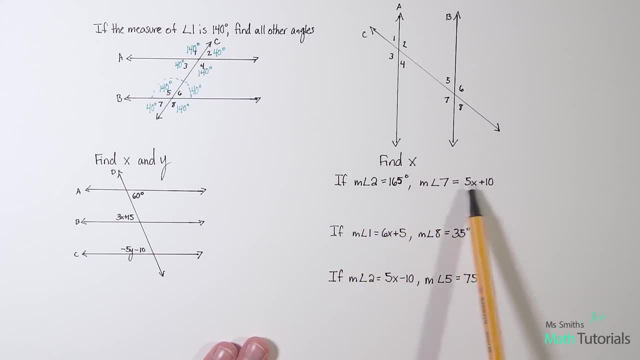 Okay, I don't take that and then build on it. It's just for this problem. Imagine that was true. Okay, For this problem, we'll have a different, a different um number that we're working with. Okay. 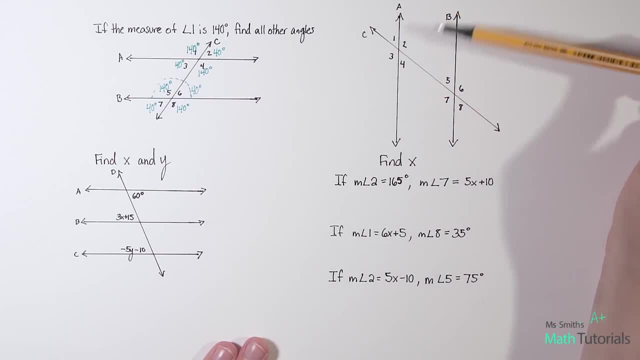 Um, so let's see. So I see that I've got A and B here, Okay, And we are operating under the assumption that these are parallel lines and I see C is a transversal that cuts through them and that creates all kinds of angle relationships. um, 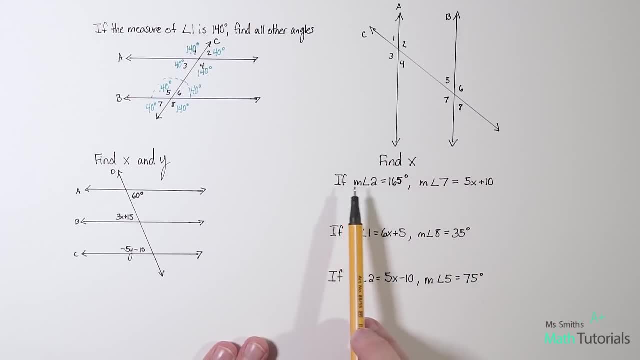 that I can build on. So for this first one, it says if the measure of angle two is 165 degrees, and it says the measure of angle seven is five times X plus 10.. Okay, So what I need to recognize is What is the relationship between two and seven? 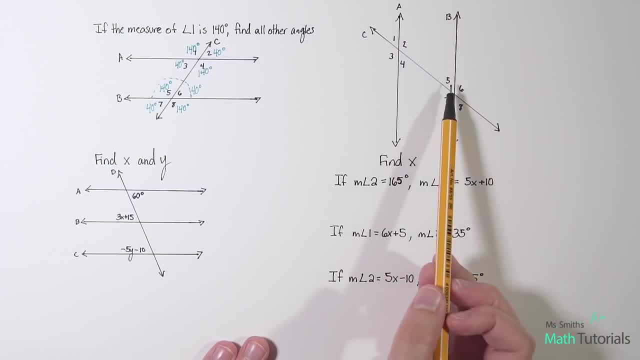 Well, they're on the interior side of these parallel lines- See on there on the inside, Okay, And they're on opposite sides of that transversal. So that tells me these are alternate interior angles. And what do I know about alternate interior angles? 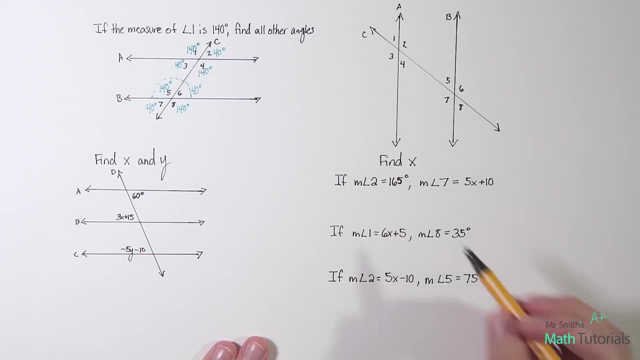 Well, they're congruent, they're equal to each other. So what I can actually do is take this uh measure of angle to 165.. And I can set it equal to five X plus 10.. Now, at this point this is just a basic algebra problem that I need to solve for X. 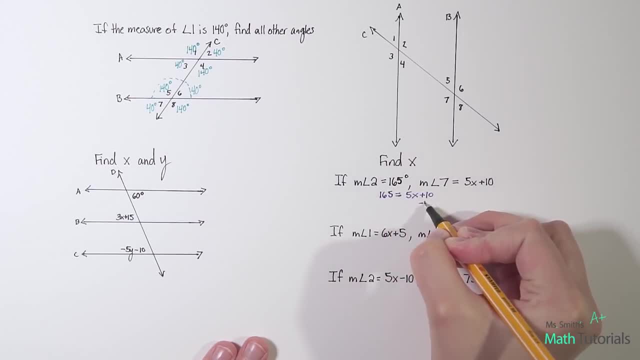 Cause that's what it wants to know. Find X, So in this case I would subtract 10.. I'd get one. 55 equals five X. Of course I want to divide both sides by five, So I know X equals 30 one. 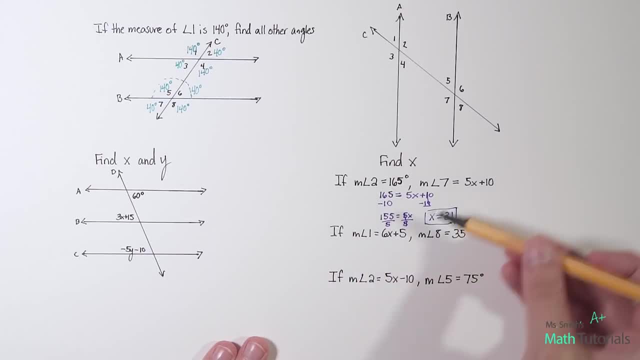 All right, Now let's um, let's look at the next one. Okay, So again, this is a totally different. we're getting rid of that 165,. moving onto a different problem, Okay, For this one. it says the measure of angle one is six X plus five. 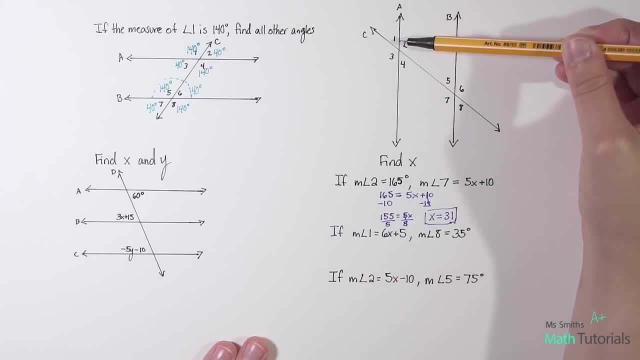 So we're right here at angle one. The measure of angle eight down here is 35 degrees. So let me see What is the relationship between One and eight. Well, I see they are on the outsides right Of the parallel lines and they are on opposite sides of the transversal. 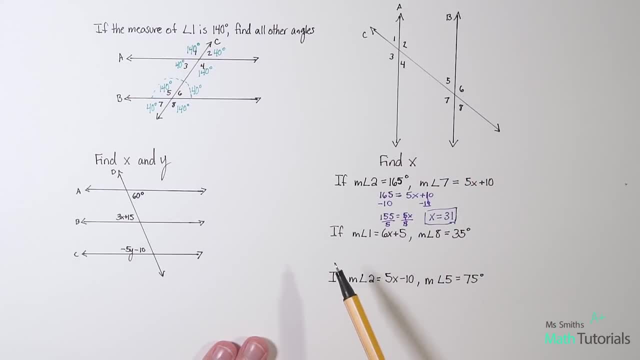 So that tells me these have to be alternate exterior angles, or on the exterior, the outside. So to solve this, I know that alternate exterior angles are congruent to each other. They're equal. So I can set six X plus five, Equal to. 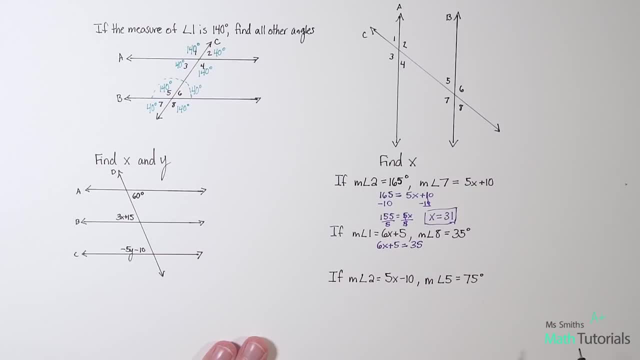 35, and let's solve for X. So I don't want to subtract five from both sides and I would get six. X equals 30, right, We'll divide by six, running out of space, and we get X equals five. Let's try this. 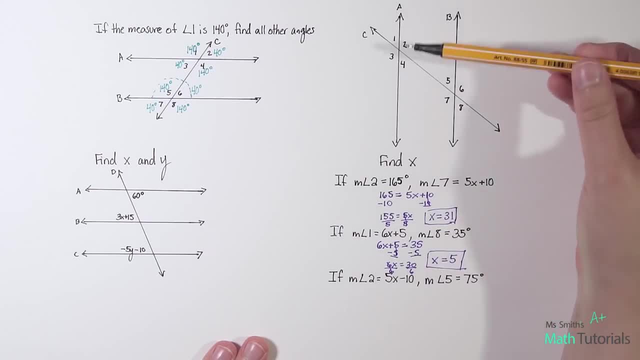 Last one, If the measure of angle two. so we're right here at angle two. measure of angle two is five X minus 10 and the measure of angle five is 75. Okay, So what's the relationship between angle two and angle five? 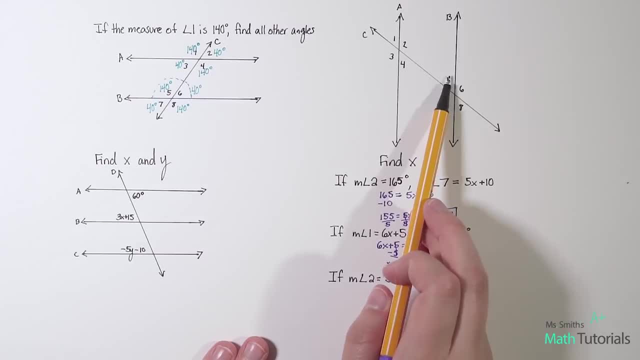 Well, I see they're both on the inside of the parallel lines and they're on the same side of the transversal. So I've got to think back. Those are consecutive. interior angles are consecutive, They're right beside Each other and they're both on the inside right. 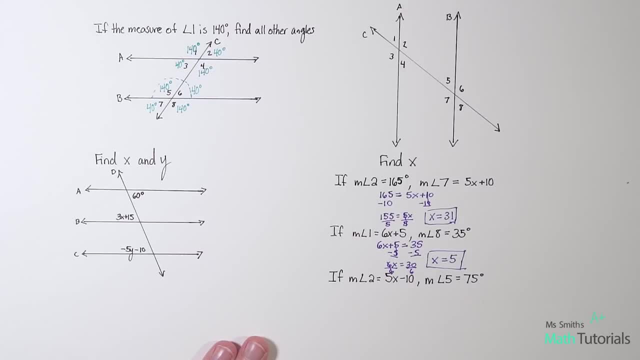 And I got to remember what's the relationship between consecutive interior angles, and they add up to 180 degrees. So this time I'm not going to set them equal to each other like I did the other ones. They're not equal, right, I can clearly see two is an obtuse angle and five is an acute angle. 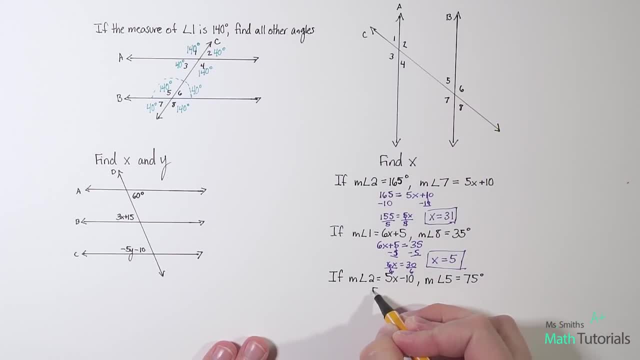 They are not equal. Okay, So I can say five X minus 10.. Plus 75.. That's going to give me 180 degrees, And now I can solve So negative 10 plus 75.. That's going to be 65.. 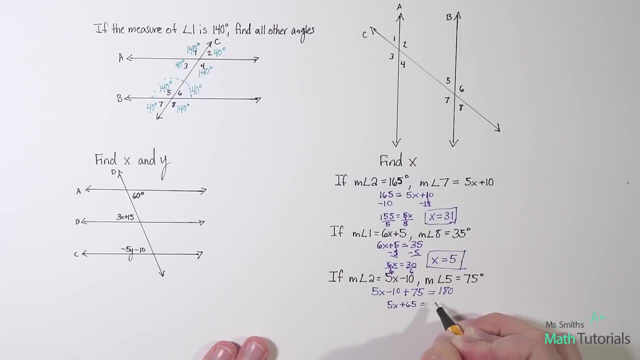 So I've got five X plus 65 equals 180. subtract 65 from both sides, That would be 115.. So five X equals 115.. Of course we divide by five on both sides and we get X 23.. Let's look at this example. 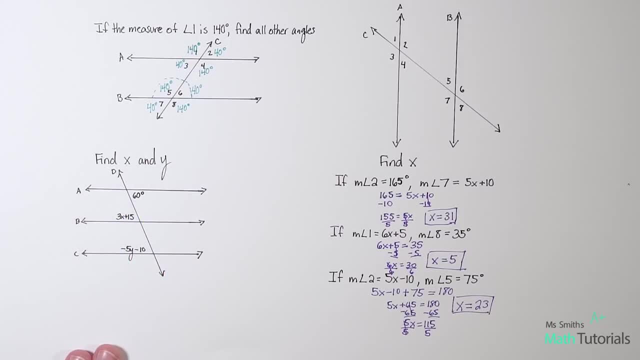 This one asked me to find X and Y, So I'm going to have to find two different variables for this problem. Looking at this, I see that I have a series of parallel lines. This time I have three lines instead of just two. 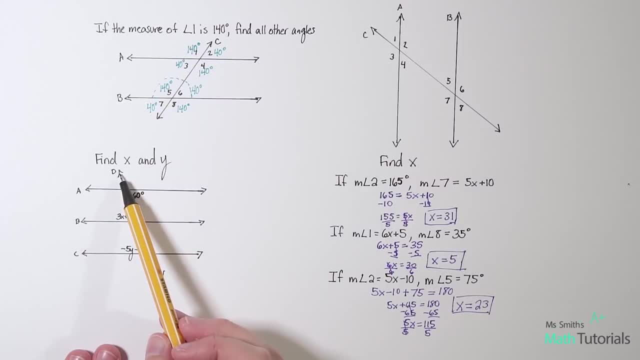 That's okay, The same rules still apply. And then I've got a transversal cut between them, line D. So I know that this angle is 60 and this angle is three X plus 15.. I'm not going to worry about the Y yet. 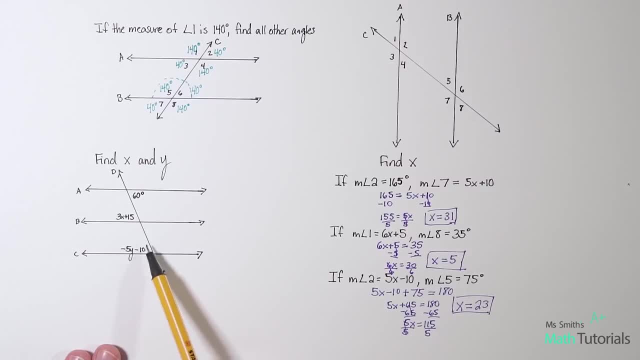 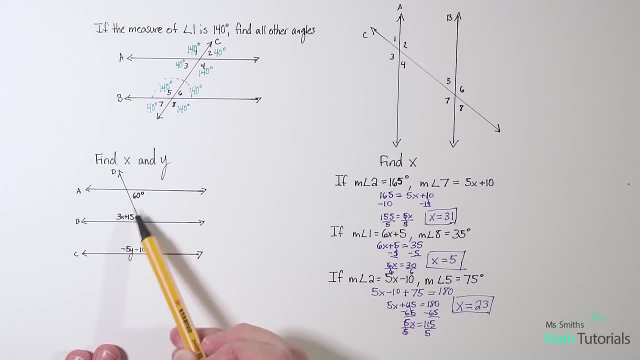 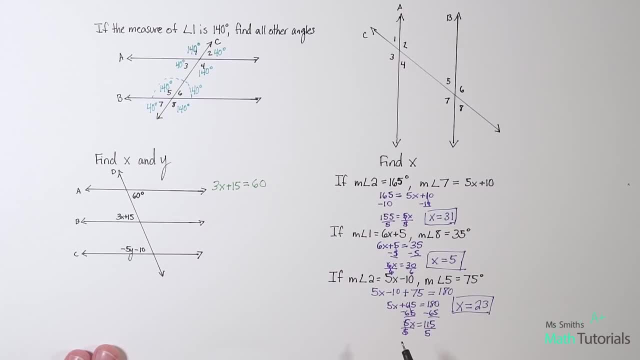 angle 60. okay, so I'd want to subtract 15 from both sides: 60 minus 15, that's going to give me 45, so 3x equals 45, and then, of course, we divide by 3 and we get X equals 15. now it's important to note, and I wish I had noted this over here as 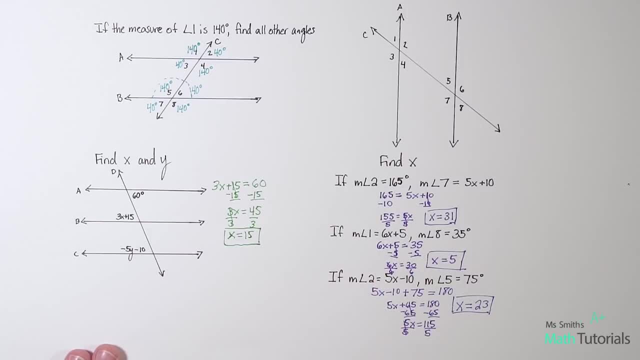 well, but it applies to both problems- that when we're finding X here, I'm not saying that this angle is 15 degrees. that's not what that means. I'm not saying that this angle is 15 degrees, that's not what that means. I'm not saying that this angle is 15 degrees, that's not what that means. 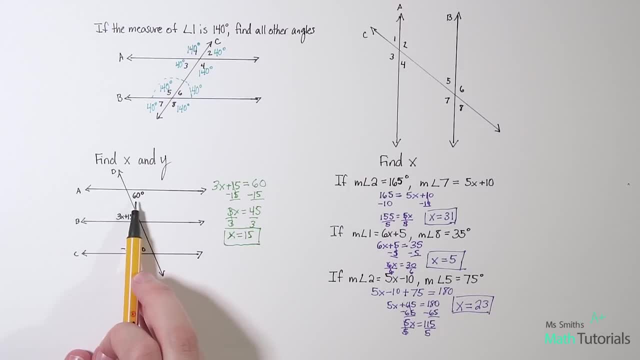 the angle itself, I know, is going to be 60 degrees. right, because these two are congruent. if this one's 60 degrees, so is this one. but what I just want to know is the value of X. so, assuming that I've done my work right, I should be able to. 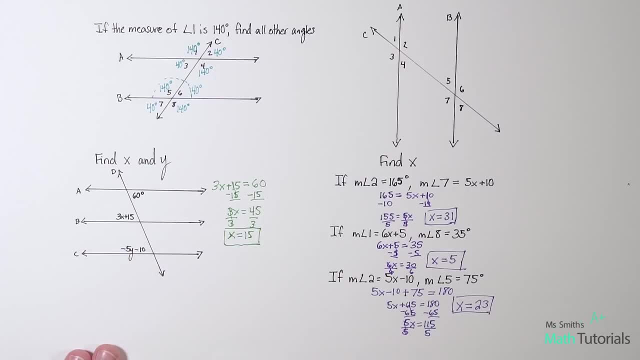 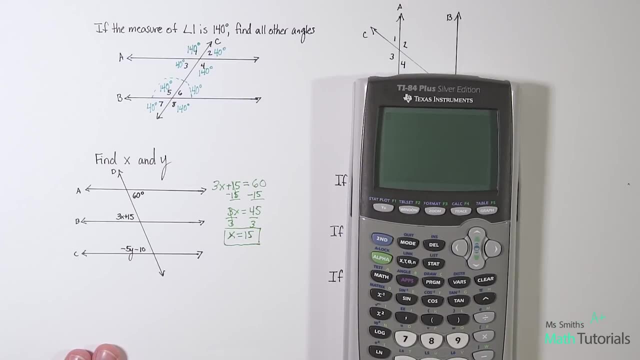 plug that X in right there and get 60 degrees. so let's just double check that on the calculator. it's good to check yourself every now and again and make sure you're you're doing the right thing. so we would do 3 times 15, 3 times X. 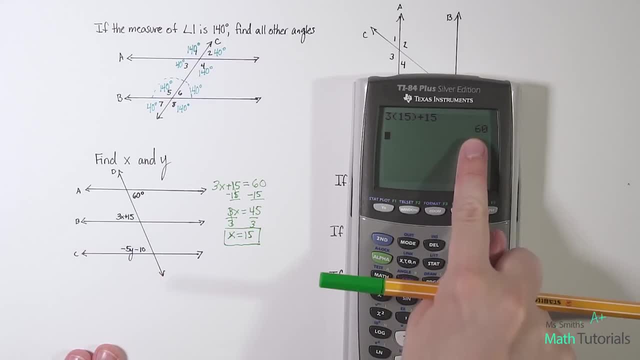 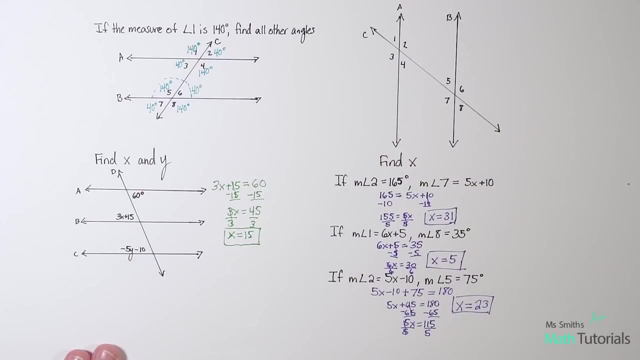 plus 15, and I do get 60, so I can feel confident. okay, 15 is right, because if I didn't get 60, that means I've done my math wrong. so good to always double check yourself. and now I can focus on the Y. I found X, now let's find Y, so I. 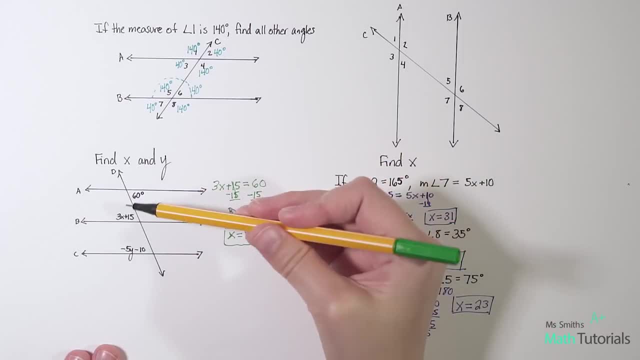 could go about this two different ways. I could either take my knowledge of this angle and apply it to this angle, or take my knowledge of this angle and apply it to this angle. I'm gonna go with this six angle and apply it to this angle. I'm gonna go with this six. 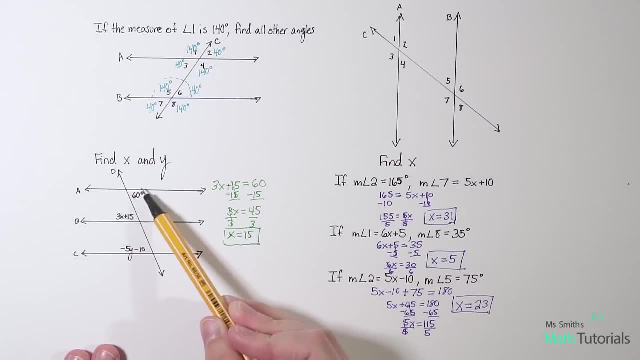 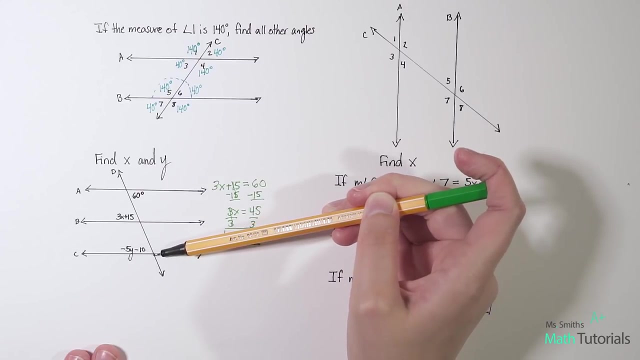 just because I think it's easier, less solving involved. it's already a whole number. So if this angle is 60, what's the relationship between this one and this one? Well, now, looking at the parallel line A and the parallel line C, these two are also on the interior when we 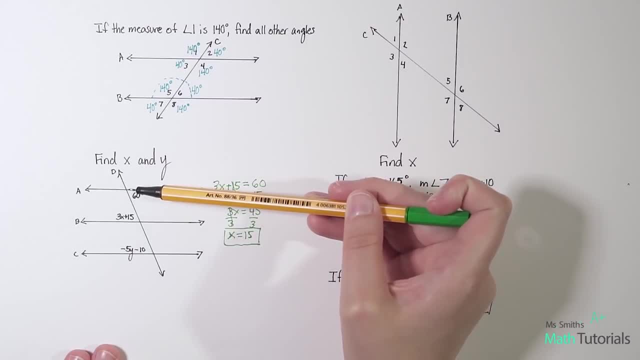 widen our scope. So for the first one, these two are on the interior of A and B right. But now we're looking at A and C and these two are on the interior. So they are just like these two. these are alternate interior angles which we know are congruent, So I can kind of do the exact. 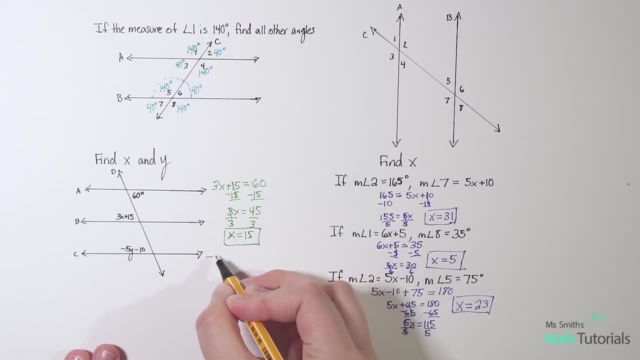 same thing again, only this time I'm going to say my y angle: negative 5y minus 10 equals 60. And now we solve: Add 10, so I get negative 5y equals 70, divide by 5, of course negative 5,, excuse me. 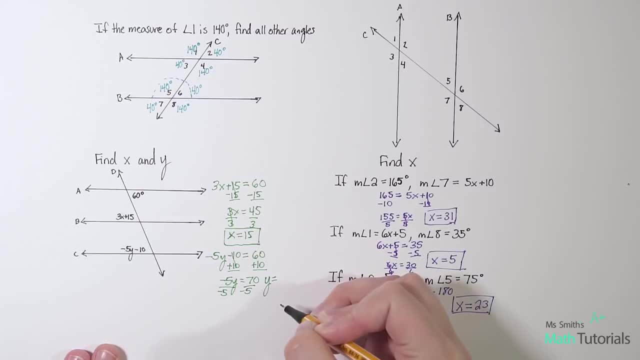 and we get: y equals 70 divided by negative 5 is negative 14.. Now this raises an interesting question. Could I have a lot of students will they'll solve a problem like this and then they raise their hand they'll say to me: well, you can't have a negative angle, okay. 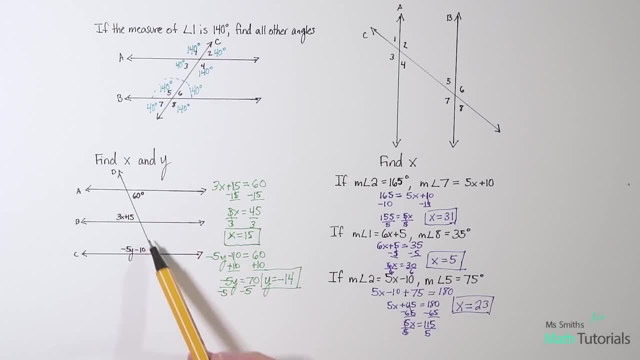 And that's true. all right, If we're doing like real life problems like this and you get a negative for an angle value, that's not good. That means you've done something wrong. okay, We don't have a negative measurement of something, But it's okay for a y or an x or a variable you're solving for.